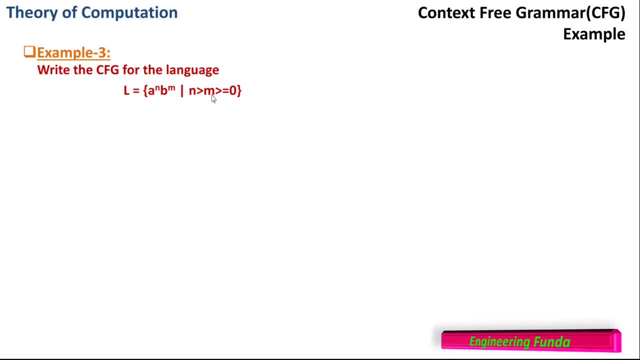 So the minimum value of m is 10.. Then the value of n can be greater than or equal to 11.. So we have to do is we have to do a function to solve this. So we have to do a function to solve this. 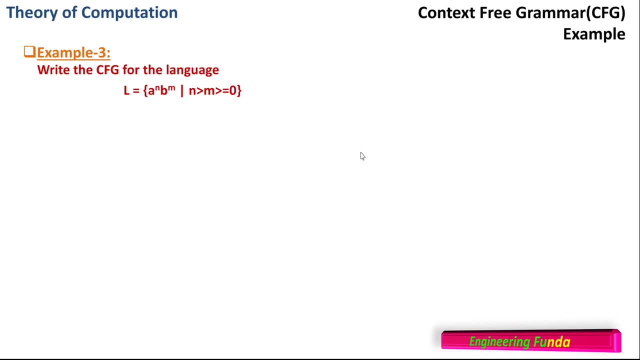 to split this condition into two parts and observe if we can find some pattern and use an existing grammar to generate the grammar for the given language. In the language asked, there are two relations to be maintained. This relation are independent of each other. This relations, like n is greater than m and m is greater than or equal to 0, are independent. 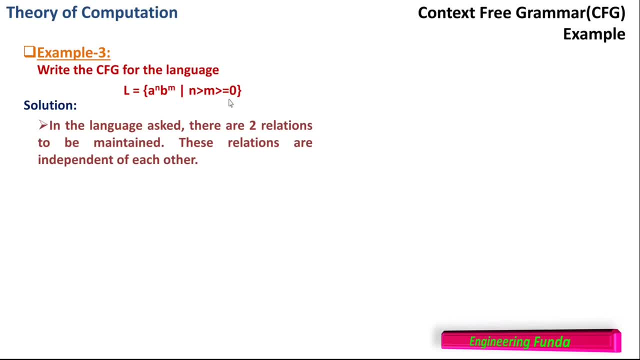 of each other, So I can divide this condition into two parts and work on them separately. This relations are: n is greater than m and n and m both are greater than or equal to 0.. This applies to both n and m, but since first condition is also applied, 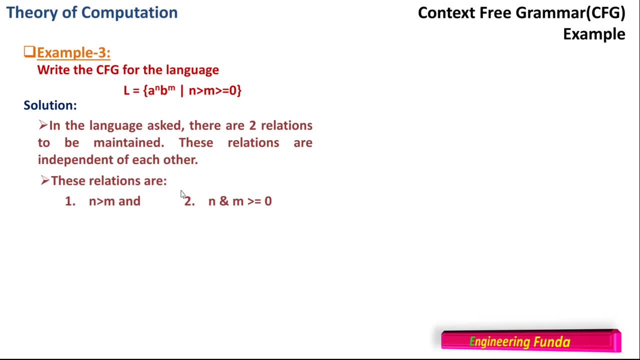 That is, n is greater than m, so my n should be greater than 0.. Here n is greater than m. can be replaced by n equal to m plus some value k, which is greater than 0.. Just as I have said in the beginning, that if my m value is 10, then my value of n is: 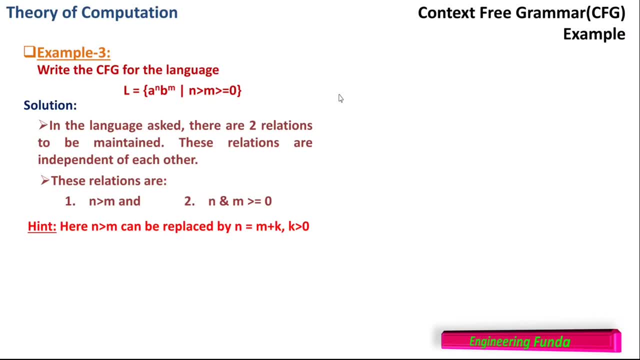 equal to greater than 0. So my k value is greater than 0, so it is at least 1.. So if my value of m is 10, then it should be at least 1.. So my minimum value of n is 11, but then it is greater than 0, so it can be 11, 12, 13, depending. 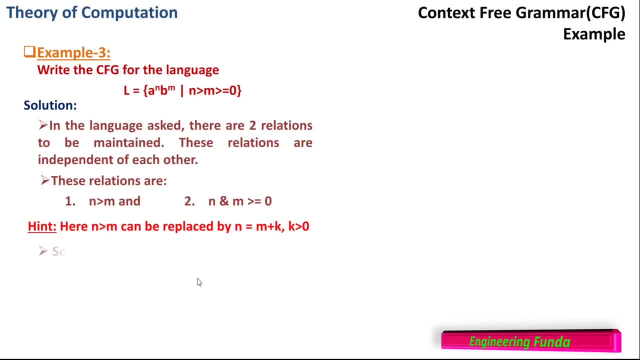 on the value of k. Now, why are we doing this? Let us see that in the next step. So we can write This language, l, which is equal to a raise to m plus k. so I am substituting this n equal to m plus k, so my n is now m plus k, so it is becoming a raise to m plus k, b raise to. 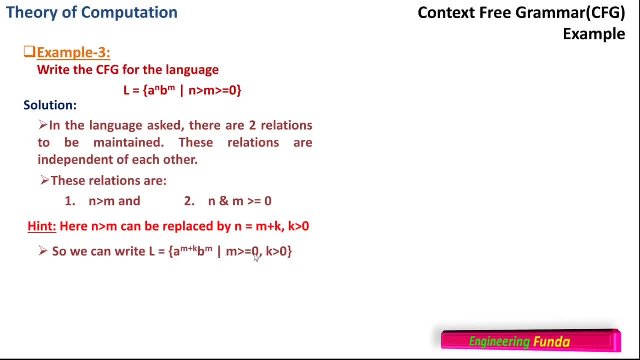 m, such that my m is greater than or equal to 0 and k is greater than 0.. So here my this two conditions which are dependent on each other: n is greater than m and n and m are greater than or equal to 0.. 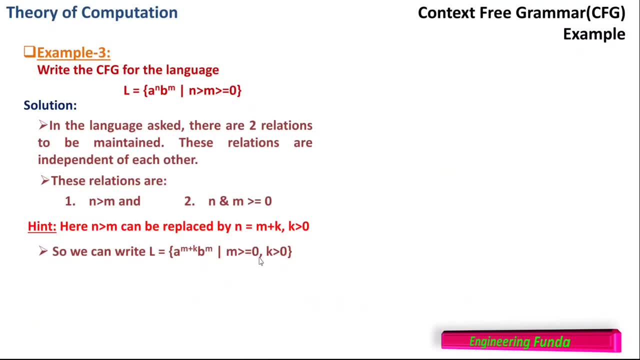 So here there are two conditions: are now getting independent. So my m is greater than or equal to 0 and my k is greater than 0. So I can rewrite this language as a raise to m, a raise to k, b raise to m. 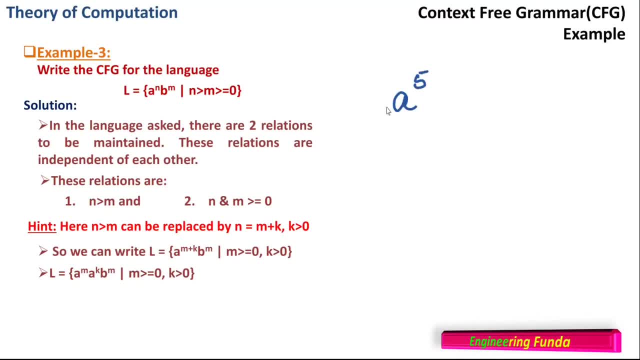 So what we can do is, if there is this a raise to 2 plus 3. Then I can write it as a raise to 2, followed by a raise to 3.. That means 2 plus 3 is 5, so it is 5 occurrences of a. that is nothing, but it is same as 2 occurrences. 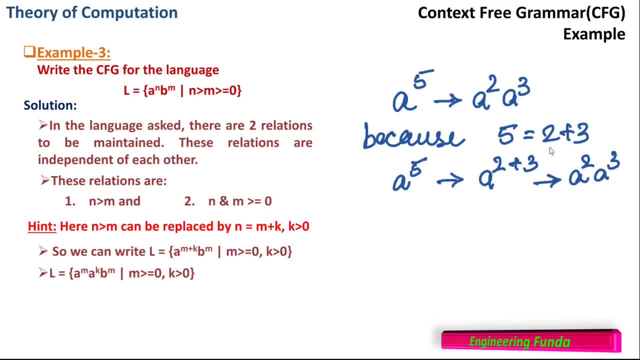 of a followed by 3 occurrences. So 2 occurrences or 3 occurrences will give me 5 occurrences in all. Hence this a raise to m plus k can be written as a raise to m, a raise to k, and this b raise to m is as it is. 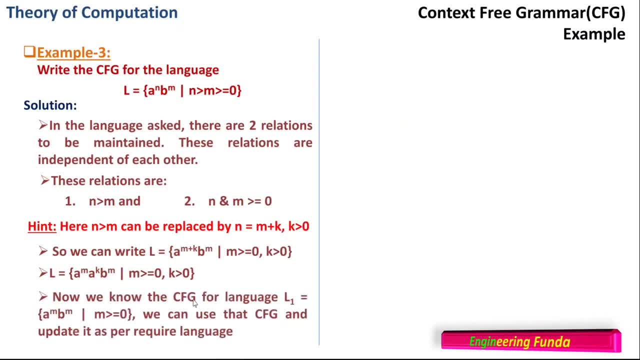 Now we know the context free grammar for the language l1, which is equal to a. raise to m, b. raise to n, where m is greater than or equal to 0. We can use the context free grammar and update it as per the required language. 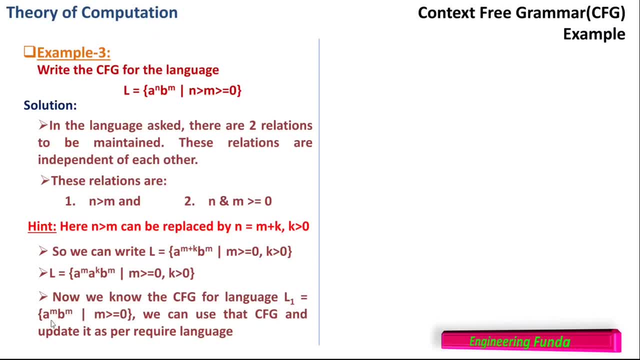 So here this language is known, where the occurrences of a and occurrences of b are same And the context free grammar for that language is already known, which is s, tends to a, s, b or epsilon. Now, if you go back to the previous video, we have seen that it is s, tends to a, s, b or a. 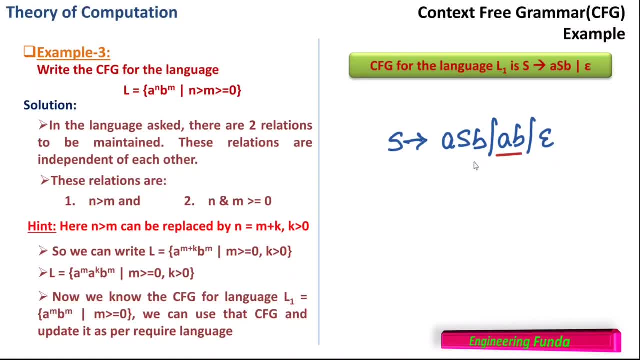 b or epsilon. Now I have removed that production s tends to a b, because s tends to a, b can be generated by using this production s tends to a, s, b and epsilon. So if I substitute this epsilon here, What I will get is a, b. 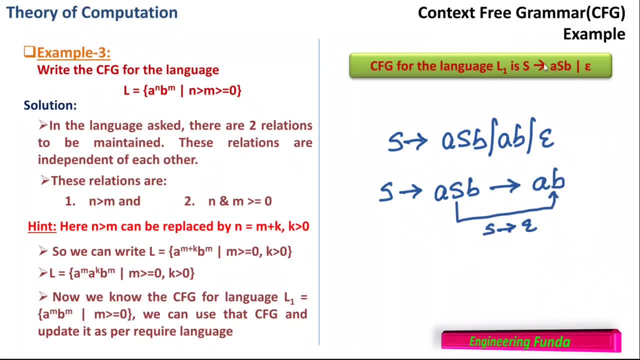 So what I am doing is I am making an unambiguous grammar from a given ambiguous grammar. So this is an unambiguous grammar for the language a raise to m, b raise to m. That means the a and b have same number of occurrences. The grammar for generation of a raise to k which is k greater than 0, is: 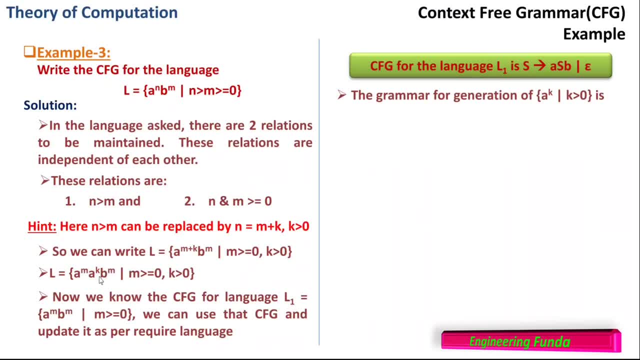 So what I am doing is- I know this a raise to m and b raise to m and this a raise to k. I will try to generate the grammar and put it into the grammar of a raise to m, b raise to m. Let us see how we can do that. 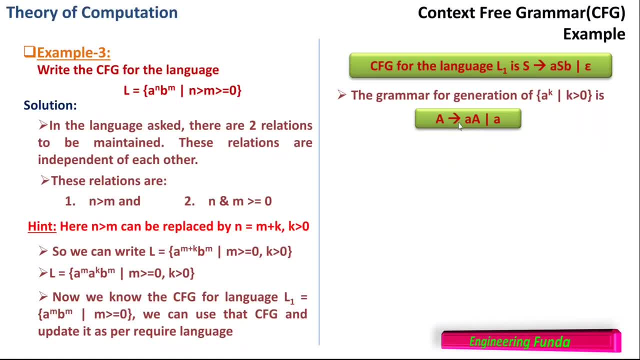 So a raise to k. k is greater than 0. we can write it as a tends to aa or a. So this is nothing, but it is a right linear grammar for generating a raise to k. We can see that for the count of a's and b's, the production a s b is used and s tends. 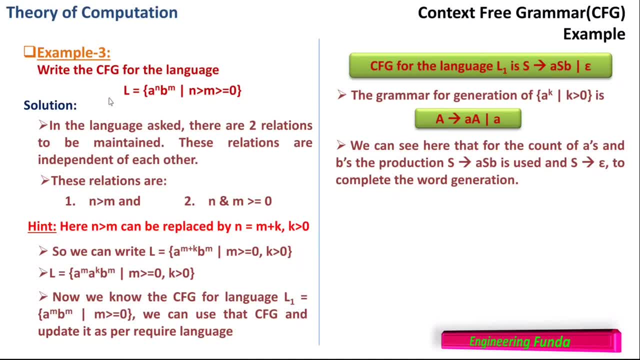 to epsilon to complete the word generation. So for a raise to m, b raise to m, the number of a's and b's are same. So we are using this a s b for the number of times we have the count of a and b and 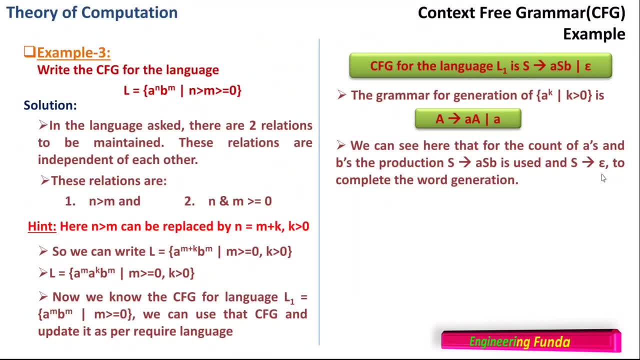 when we want to stop the word generation, We say that now the word is used, So we are using this: a s, b. for the number of times we have the count of a and b, and we have the number of a's and bs for the number of times we have the count of a's and. 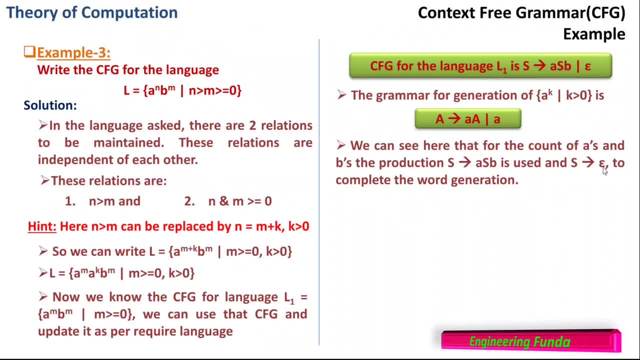 bs, So the number of a's and bs is generated. We use this production as tends to epsilon. Now, for this given language, l, which is a raise to n, b raise to m, what we have to do is the termination condition in l1 should be the point where the additional a's are added. 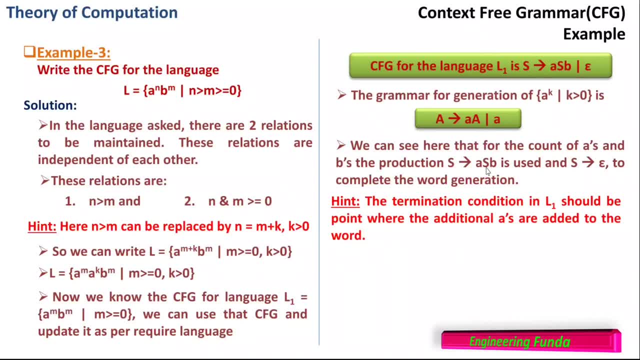 to the word. My epsilon is being substituted in the middle of a and b. To solve this function, we have to add an a to l. Let's see that of the word generation. Now, at this position, what I can do is I can focus on the additional a's.